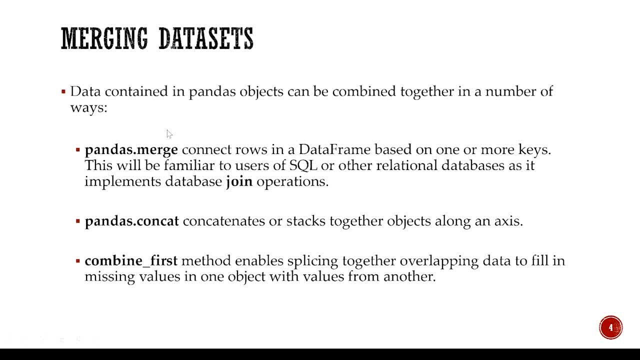 Data contained in pandas objects can be combined together in a number of ways, and you can see three different techniques here, So I'm going to go over each technique and present a few examples. The first one applies the merge method. Merge method connects rows in a data frame based on one or more keys. 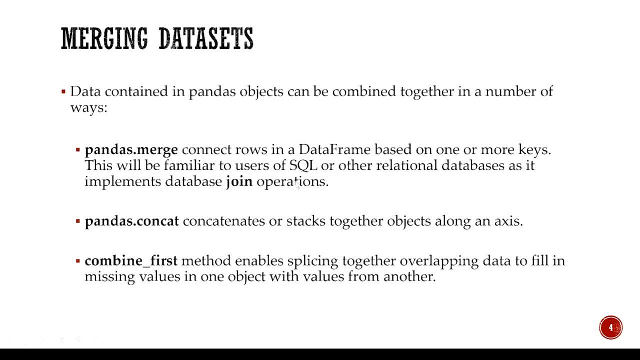 And this will be familiar to users of SQL or others- And it implements database join operations. The next technique is concatenation: Pandas can concatenate or stack together objects along an axis. And the last technique is combine- underline first method- which enables splicing together overlapping data to fill in missing values in one object with values from another object. 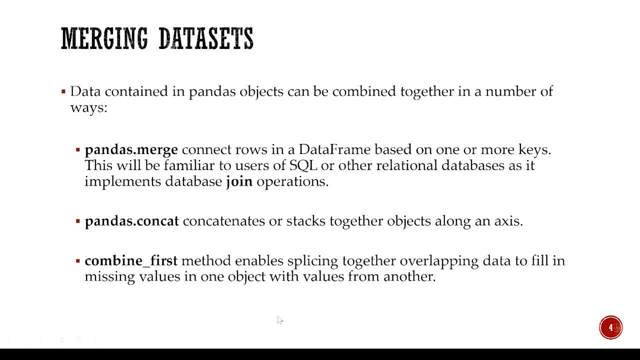 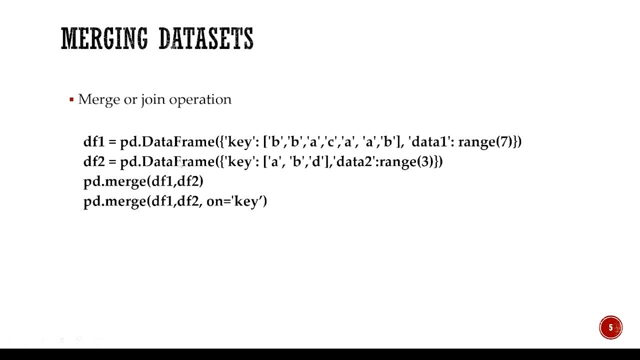 So we are done. I'm using a dataset to fill in missing value in another dataset: Merge or join operations. So in this example you see two data frames. The first one has two columns. The second one has two columns as well. 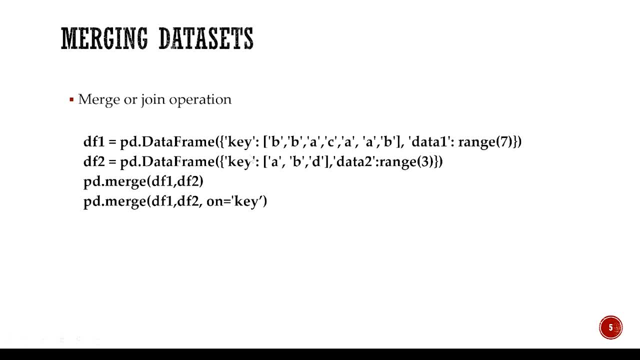 Both data frames have one common column, so key, And then we apply the merge method to merge these two datasets. First we don't specify which column we want to merge on And then, using the on keyword, we use the column that dataset can be joined on. 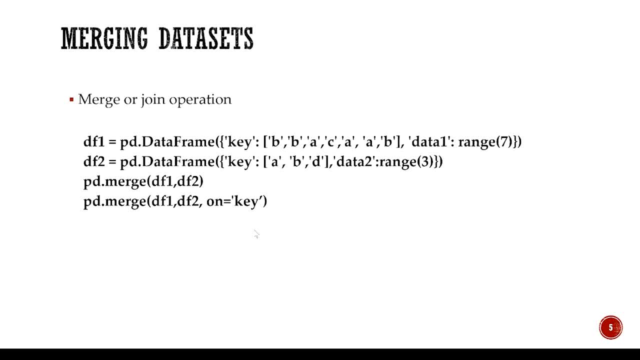 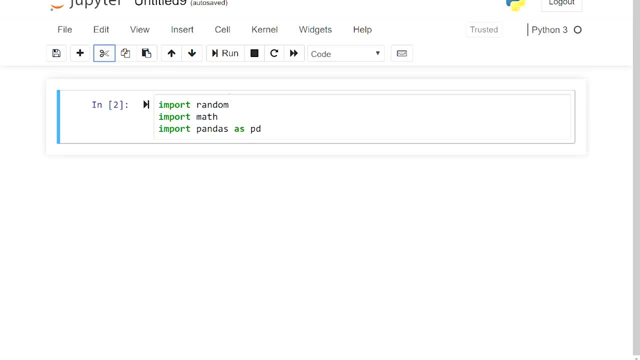 So this is an example of many-to-one join. So when we run this in Python notebook, you are going to see. So let's create those data frame quickly. So df1 is pandasjson. This is pandasdataframe Use dictionary. 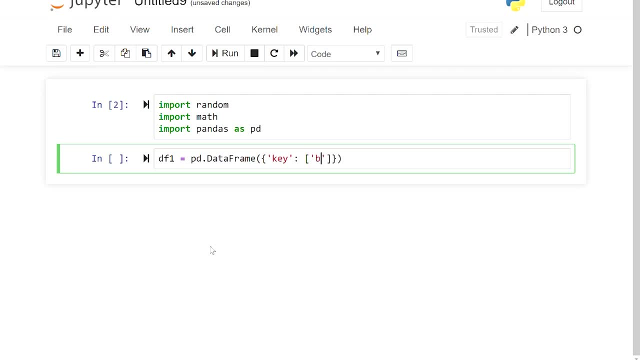 The values for the first column are two Bs, A C, Two As And one B. The second column is data1. And we use a range function to generate the list Range of seven. And if we run this And print, 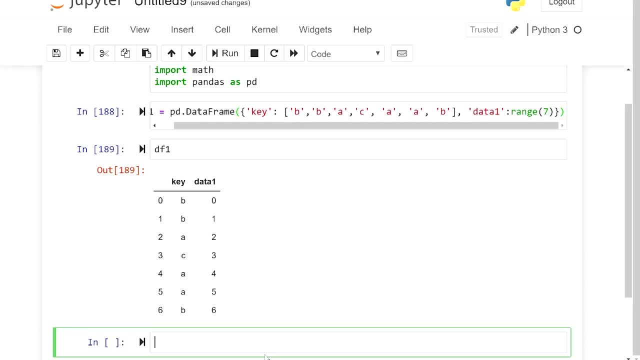 So you can see a table with two columns and seven rows. The second data frame, We use dictionary. The first column is named key And there are three rows, A, B and D, And the second column is named data2.. 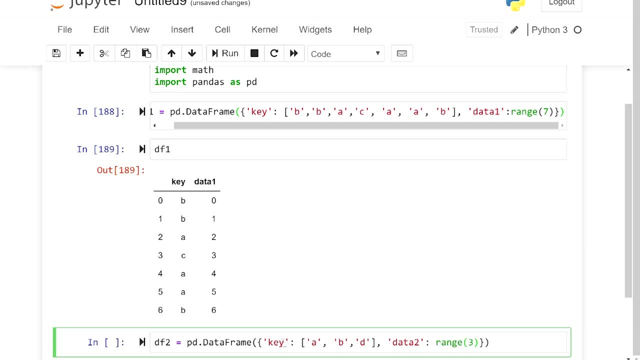 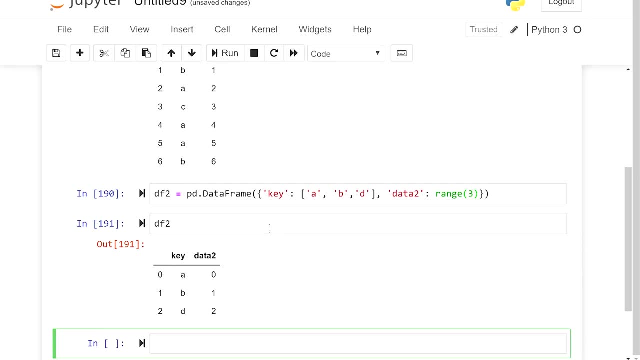 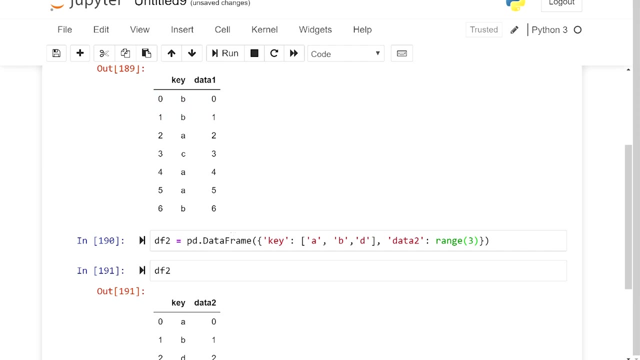 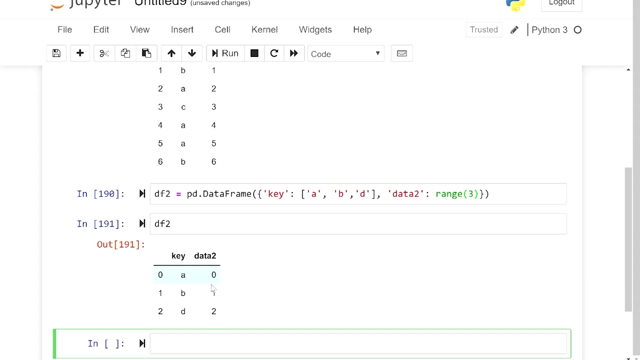 We use a range function, Range of three. So when you look at the first data frame, you can see there are several rows with B and A And if you look at the table from the second data frame, each row is unique And that's why I mentioned this is an example of many-to-one join. 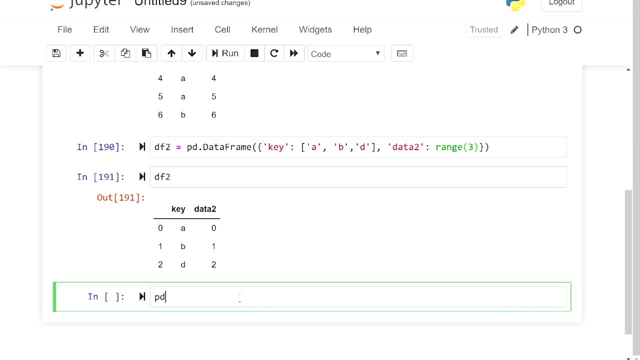 Okay, So we want to merge methods, So pdmerge, We want to merge these two data sets, df1 and df2.. And this is the result. So we can see a table with three columns: Data1,, data2.. And we didn't specify any column to join the data on. 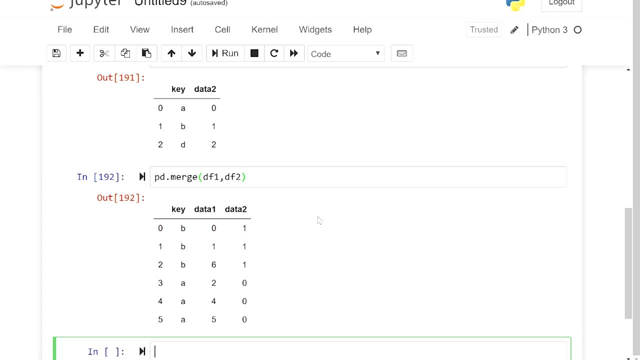 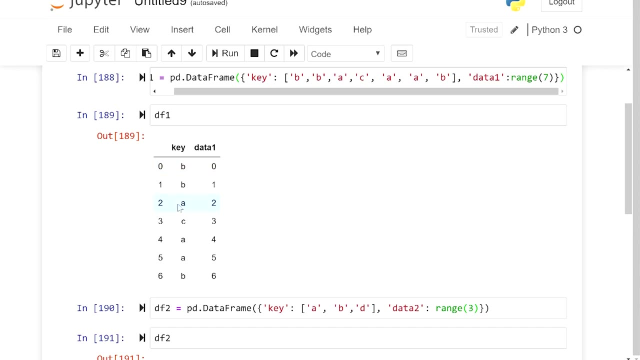 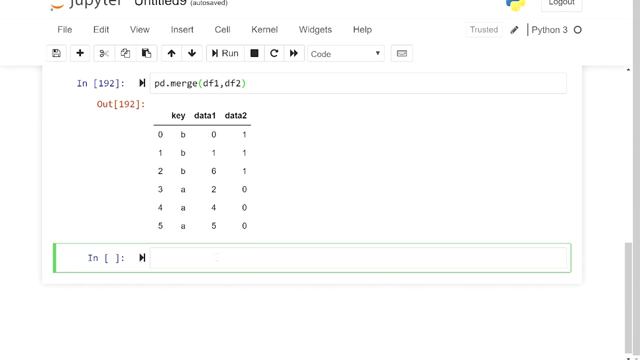 But by default Python chooses the common column. So in these two data sets we had one common column key And that's the column which is used to join or merge data here. But if we want to specify the column we can use the on keyword. 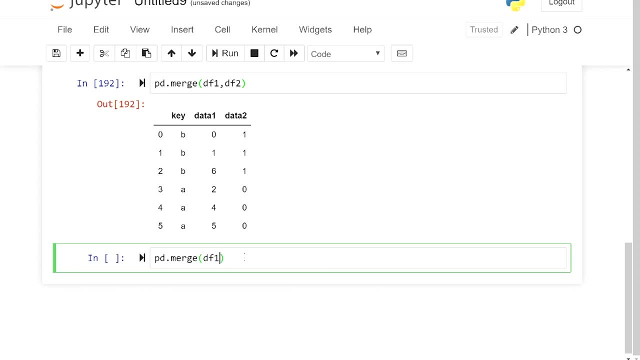 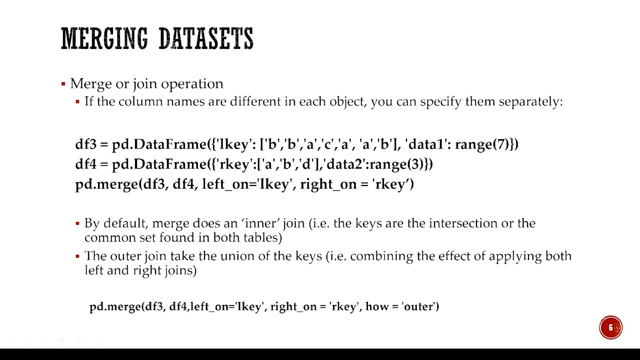 So pdmerge Again two data sets On key. The result should be the same, Because what, By default, the key column was used for joining the data? Now, if the column names are different in each object, then you can specify them separately. 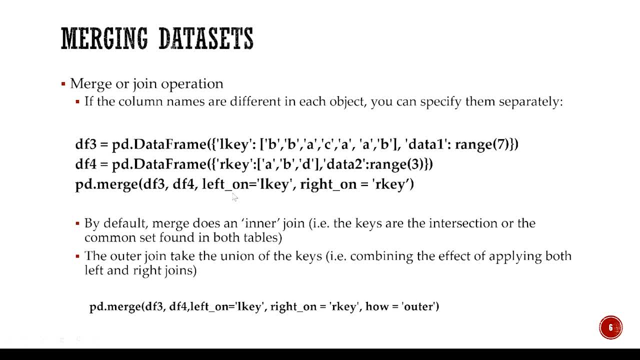 So we add two other arguments: Left underline on and right underline on. Left on is associated with the first data set, And then you specify which column, And right underline on is associated with the second data set, And then you specify the column. 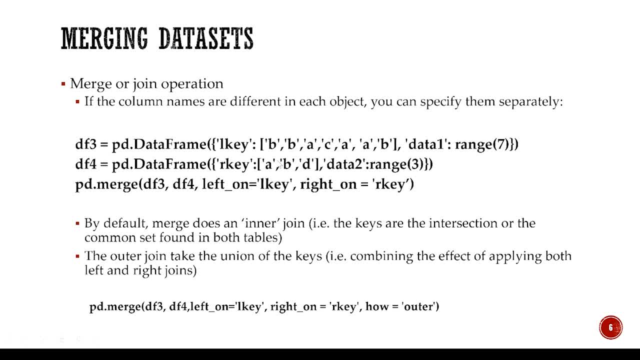 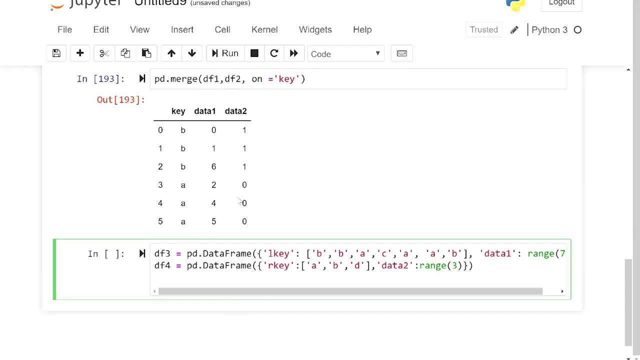 So in this example you see two data frames And there is no common column. So we pass left on and right on as statements And then we merge the data. Let's quickly see what the results look like. So first we generate the data frame. 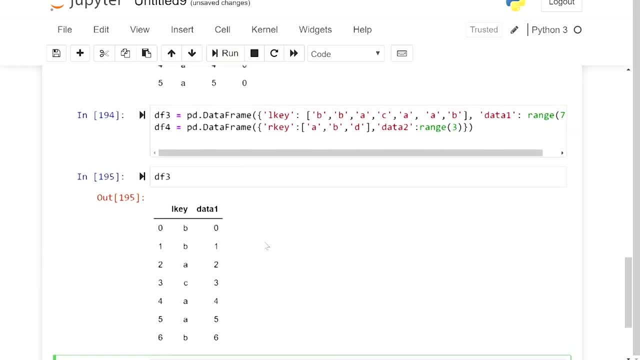 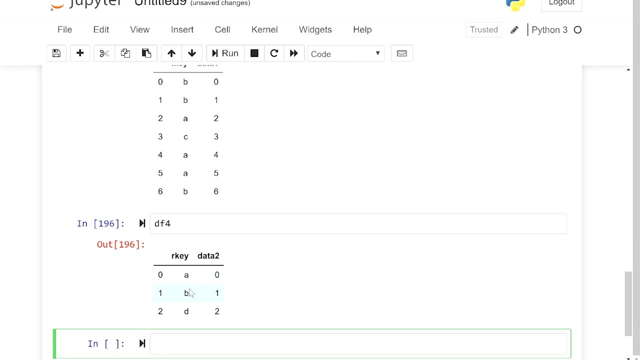 Let's take a look. So the first one has two columns, L key and data1.. And the second one. The second one also has two columns, But with three rows, And now if we merge them, These two data sets And we need to pass left on. 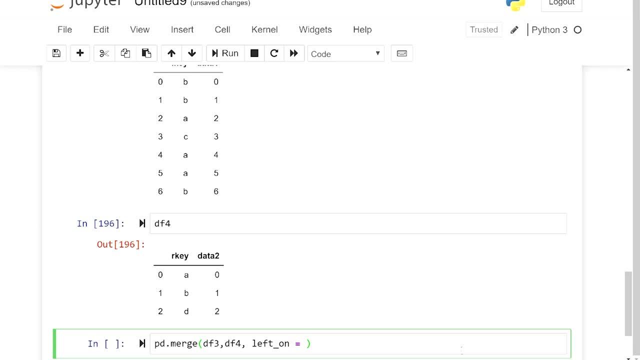 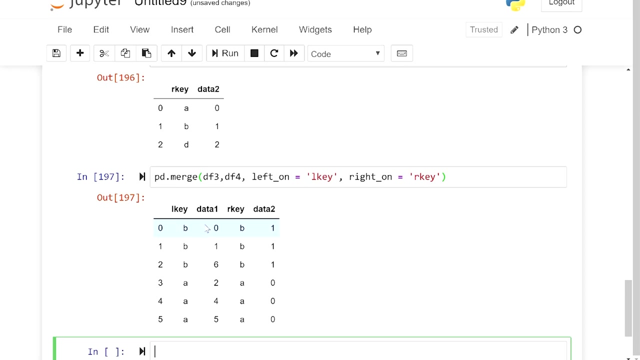 Left underline on And right underline on. So left underline on is equal to L key In this example And right underline on Is equal to R key. Now, if we run this, You can see the data frame has four columns. 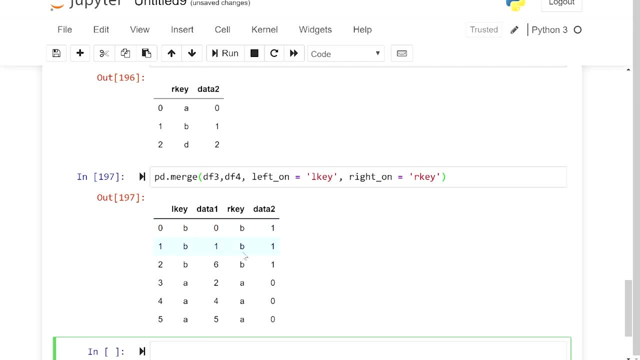 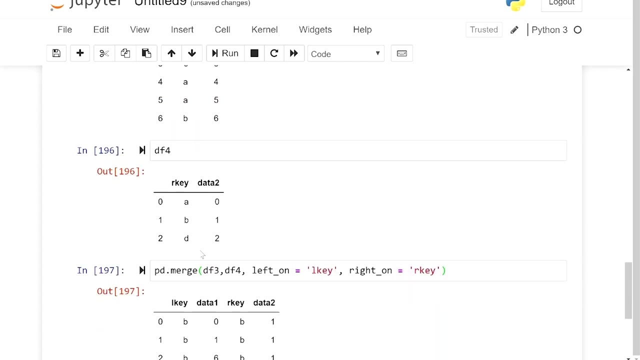 And all of them. If you look at the L key and R key columns, You can see that we only have A and B. Alright, So we C and D values, Because we had C and D in both data sets. C and D values are missing in this result. 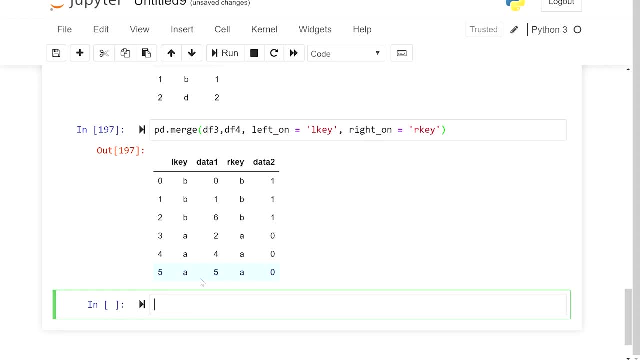 When we merge these two, It's because by default Merge function doesn't inner join. It means that it looks at the intersection of data. But if you want to have the union of your data set, Then we can pass another argument: We make it outer. 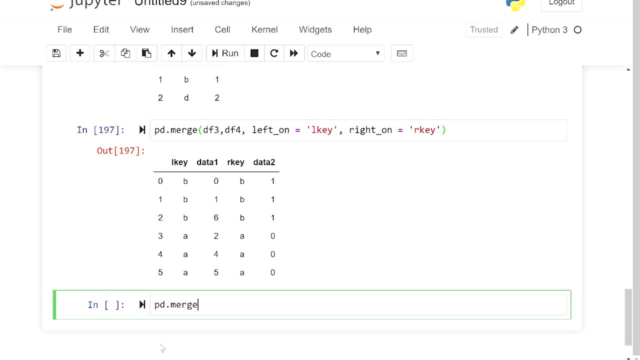 So we call pandas, We still apply the merge function To the same data set, Still we use the left on And the right on Statements, But we add another Argument, Which is how Equal to Outer. So by default, 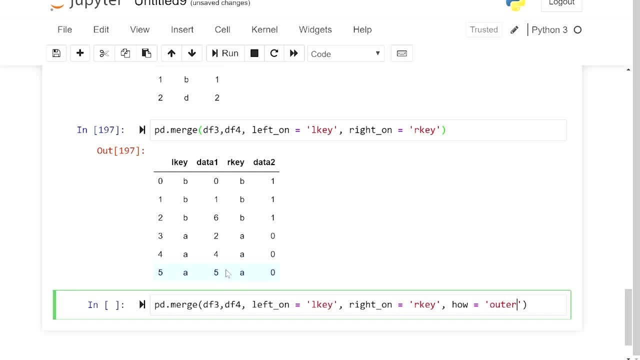 It uses The inner method. Okay, When you run this Now, You can see Data structure, A data frame With four columns, But this time Seven rows, And some of them, Some of the values, Are Missing. 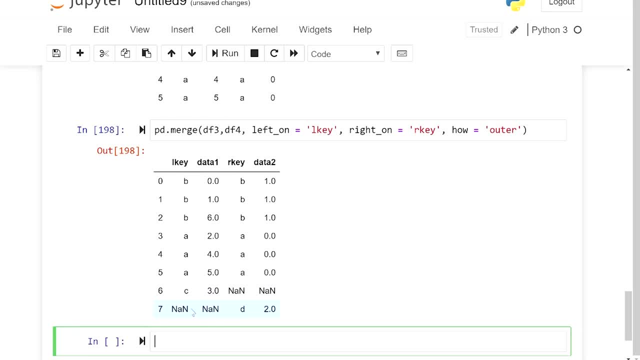 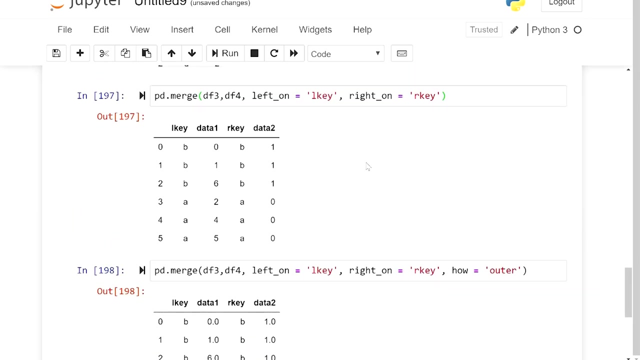 Here. So Now We can see That This Is So. It Prints The Union Of your data set, But if you don't Specify, It automatically Goes With The inner join Or the intersection. 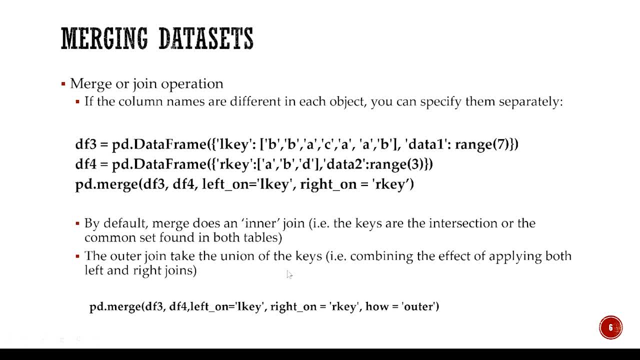 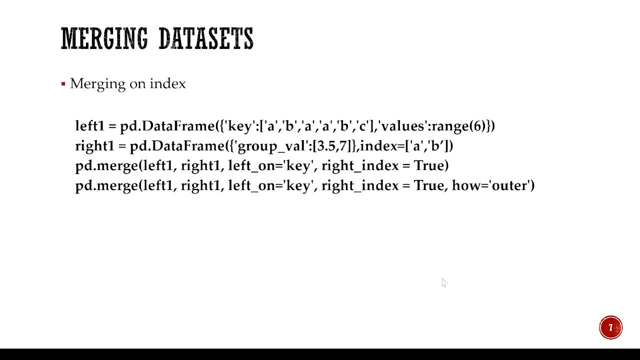 Of your data. So the inner join, The keys Are the intersection And for Outer join, Then combining The effect Of applying Both left And right Joins. Sometimes We want To merge Data set. 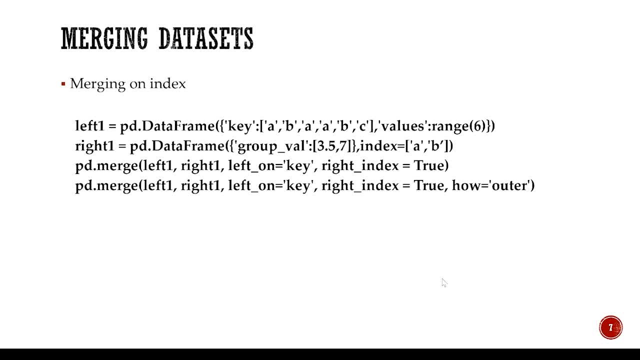 On index Data frame And index Is assigned To each row By default. It starts From zero, One And so on, And if We pass Index Argument, We can change The index For each row. 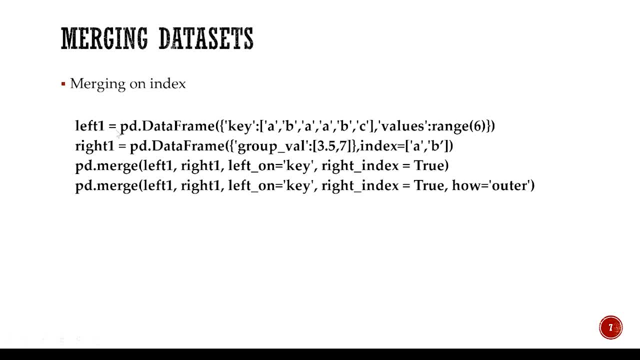 In this Example You can See That How We can Merge To Data frames Based On Index. The second One Has One Column, Group Val And Two Rows. 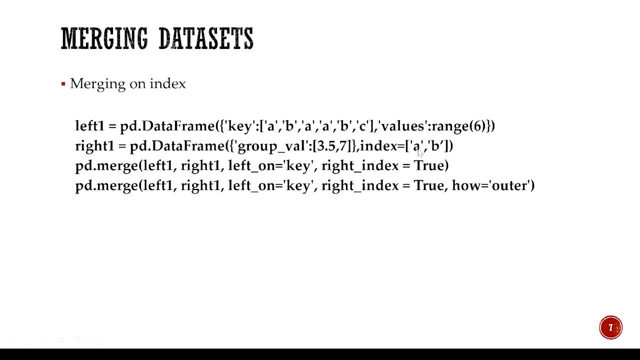 What We Assign Index To The Second Data Set. It Means That The First Row, The First Row Index, Is True And Then Right Index Equal. 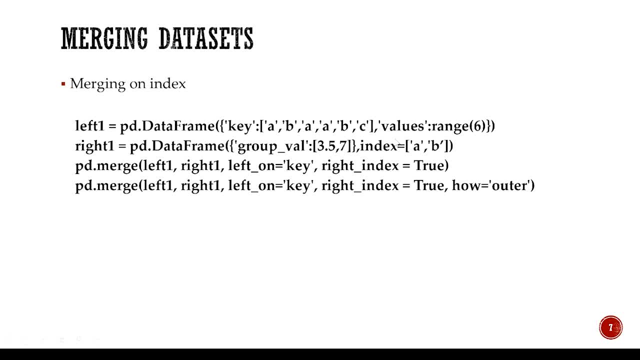 To True. So It Means That Now We Want To Merge On Index. So To Specify That You Want To Merge On Index. So Let's. 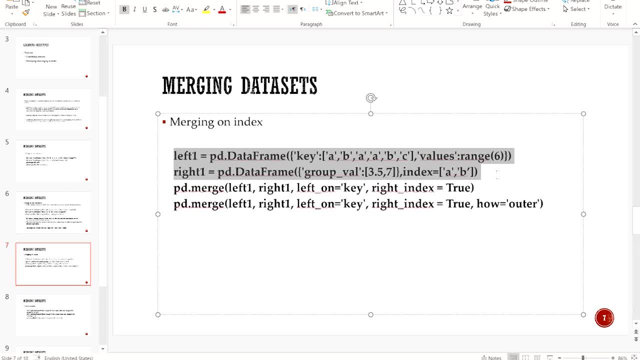 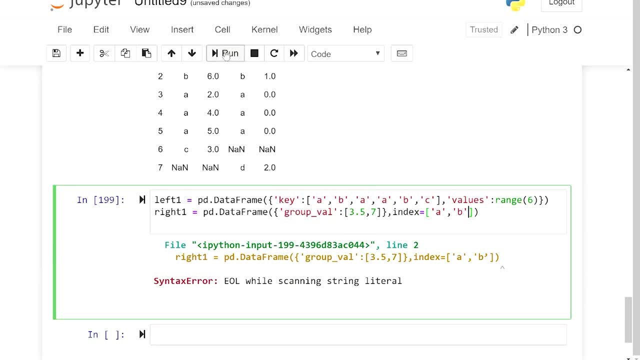 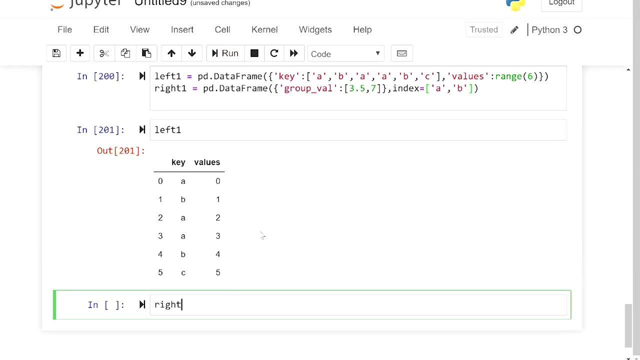 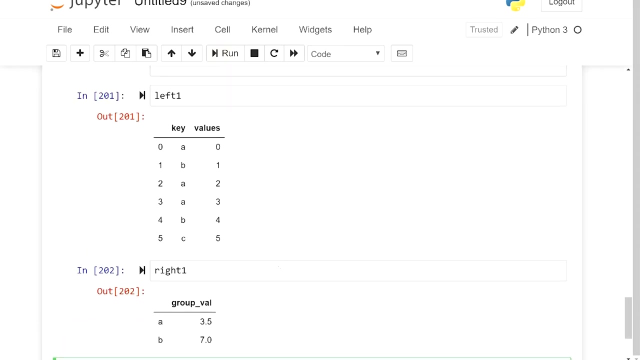 Implement This In Notebook And See How This Is Different. So We Create Two Data Frames. Let's Print Them. So Are The Original Data Frames. 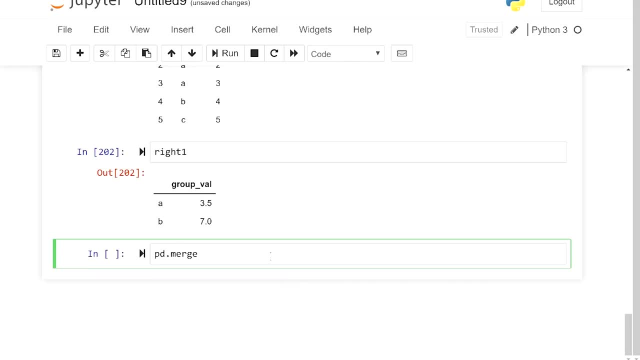 And Now We Want To Merge On Left One And Right One Data Sets, So Left On. We Want To Merge On The Key Column Then. 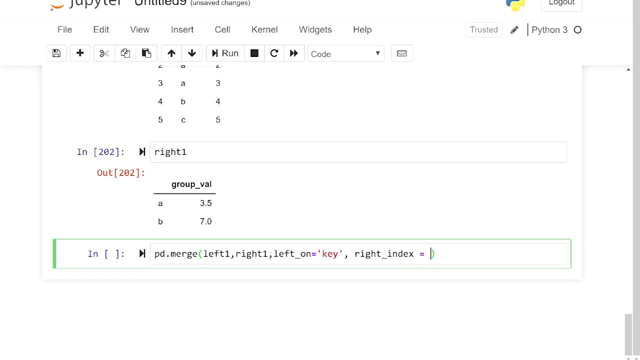 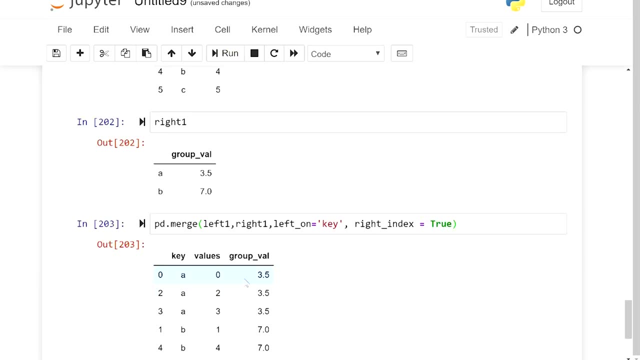 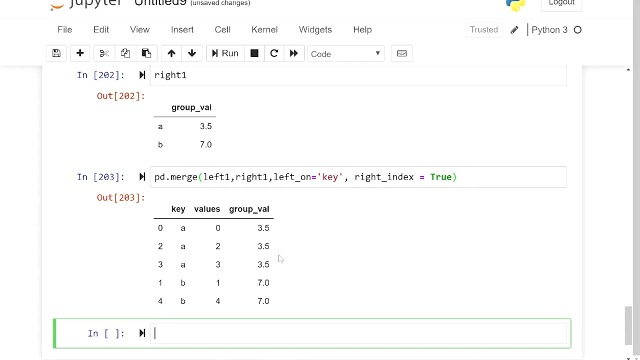 For The Second Data Set. We Now, You Can See, You Have A Data Frame With Three Columns: Key Values And Group Values. And If You 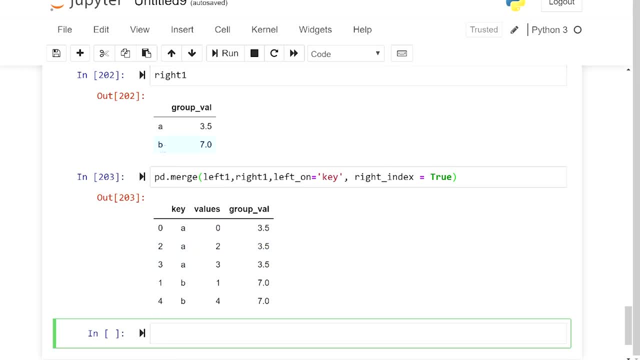 Look At The Last Column For Example For All. That's How These Two Data Sets Are Merged And If You Want To See The Result. 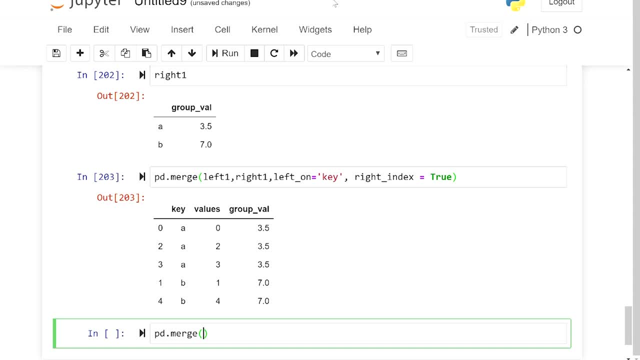 For The Outer Joint, The Union Of These Two Data Set. Then We Use The Key Column For The First Data Structure And Then We Use 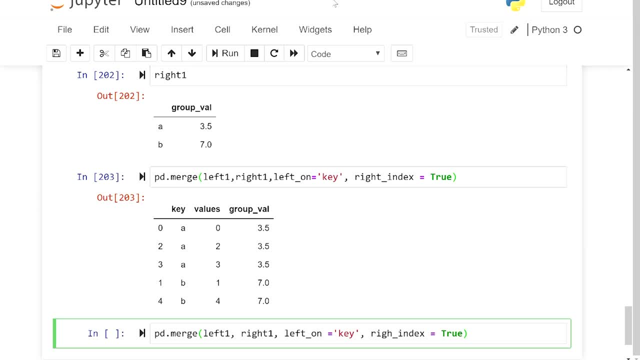 Index For The Second Data Frame And Now We Change It To Outer, There Is A. Now You Can See That We Have One Missing Value. 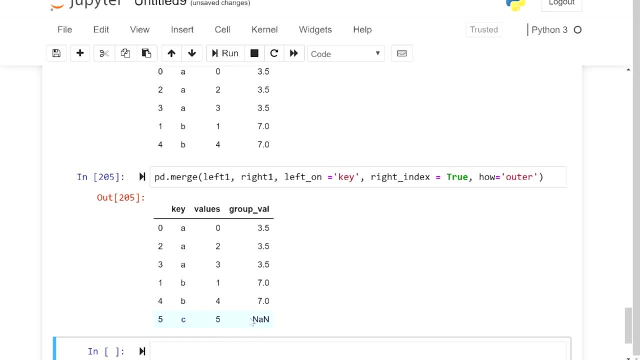 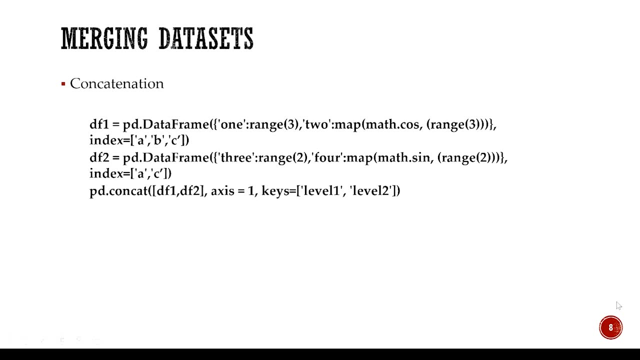 Which Was Removed. If We Go With Inner Joint, The Last Row Is Added. We Can Also Merge Data, Set Data. So If You See The 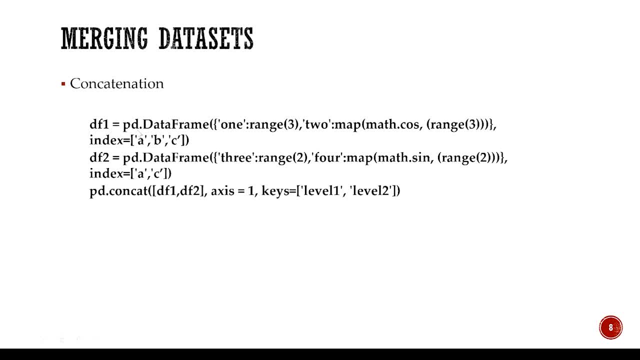 Example. It Makes Better Sense. So We Create Two Data Frames. The First One Has Two Columns, One And Two. This Time I'm Using B. 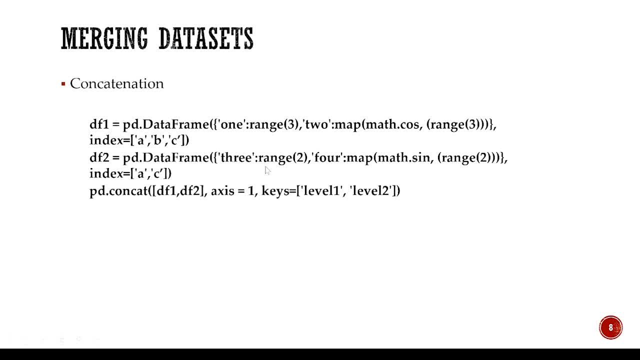 And C. The Second Data Frame Has Four Column And Has Two Columns, Three And Four, And In This Data Frame We Calculate The Sign Of. 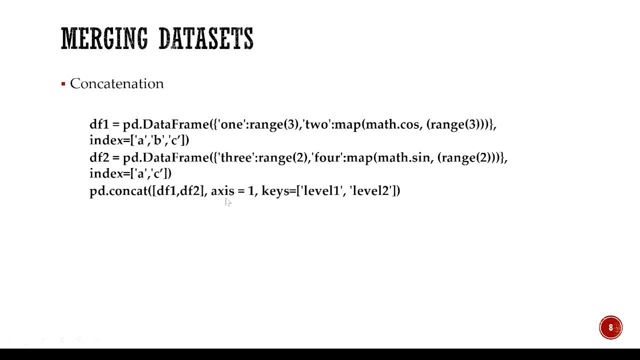 The Frame With The Column And The All The Column And Column Of The Column And The Column Of The More Scales Of Column And 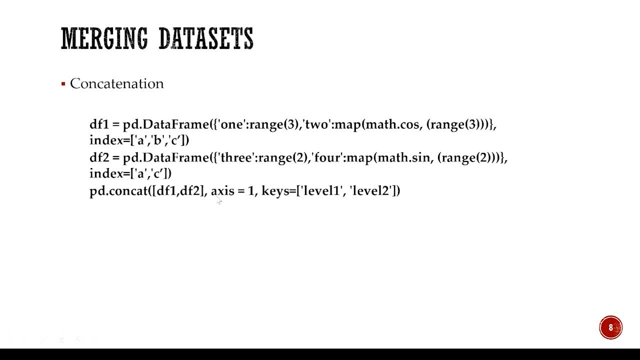 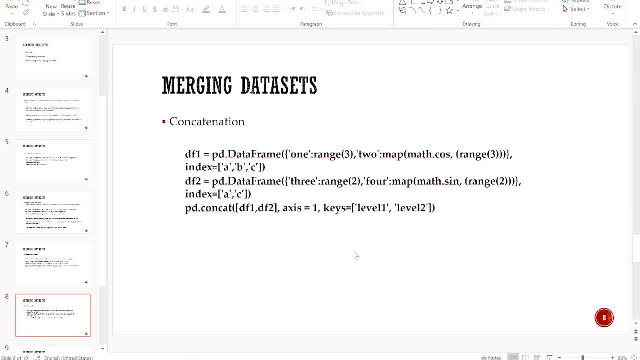 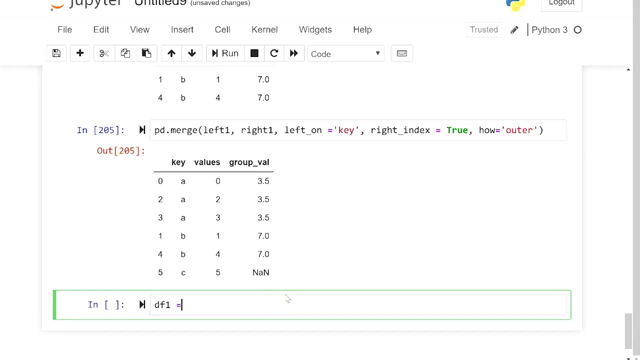 The Column In This Frame to 1. it will be assigned to rows. now let's implement this and you will get a better idea about this technique. so I create two data frames, and this is a good practice because we are using the map function. 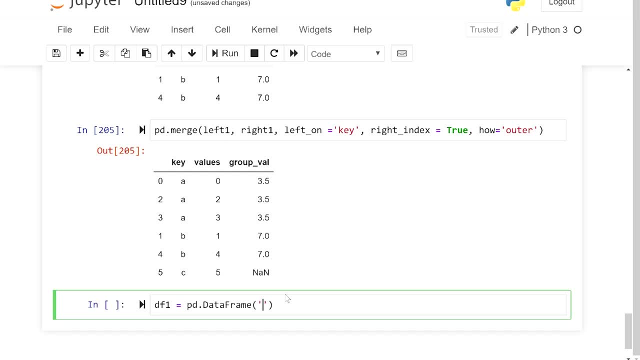 I use a dictionary in the range of three to generate values, and the second column is named two and for this one I'm using a map function and using the cosine function defined on their math module. so first it generates range of 3, which is a list as starting from 0, and then it 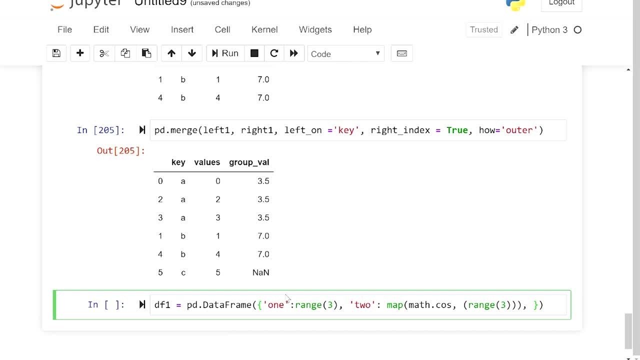 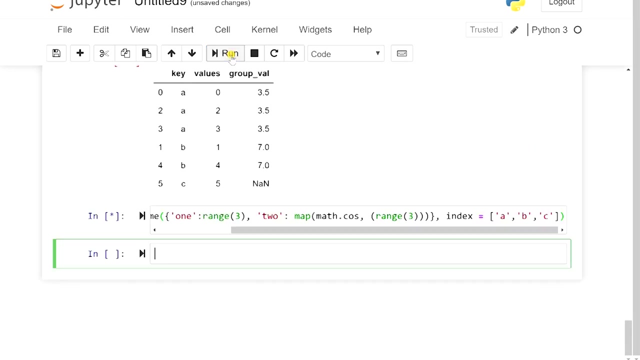 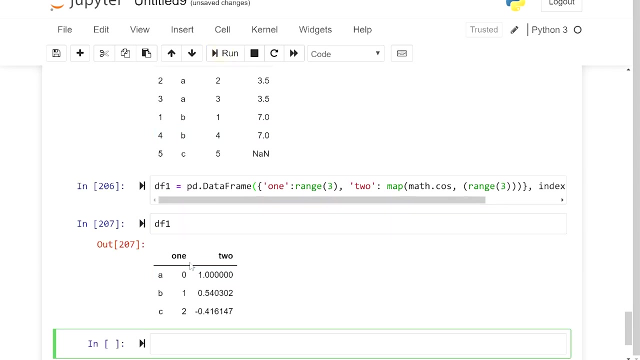 calculates the cosine of those values, and we pass index. we have three rows: A, B and C. let's run this first, let's print this and this is the result: two columns, three rows. the first one is range of 3. the second column calculates the cosine of 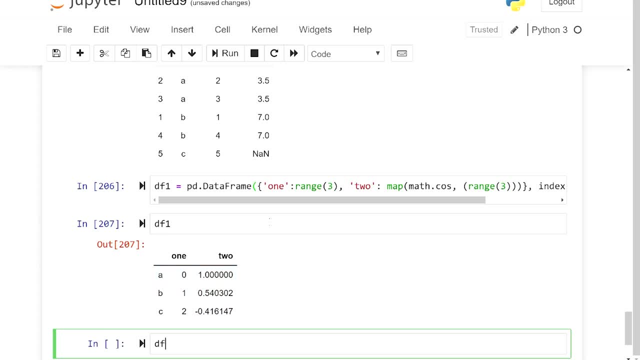 these numbers. the similar way, we can create another data frame this time. so we need to change the column names three and four. in this example, three is range of two, four. let's run it and run it: pass index and the index is negative. the second column still has. 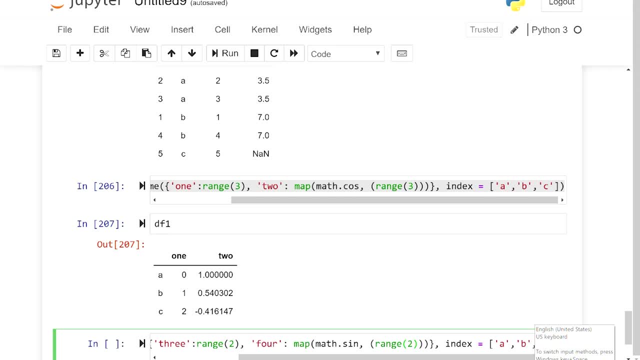 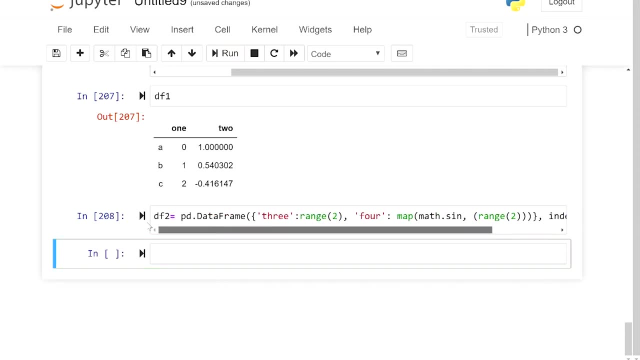 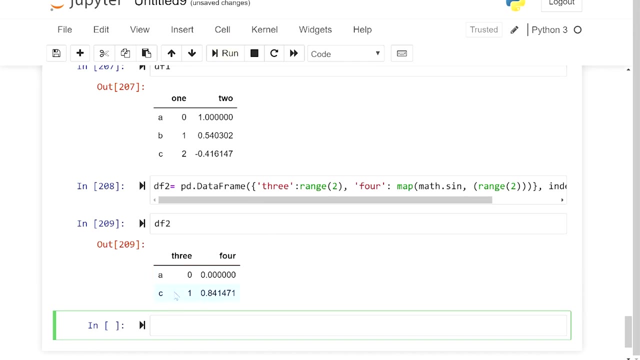 only some size. also, we now look at this labinal using a script that calculates the sine function range of 2, b pass index and the index is, let's say, a and C, because we have two rows. and then let's print this data frame so you can see a table with two columns, you can see the index for each row and again we are going to do the index. again we have two columns and again we are going to do the index. 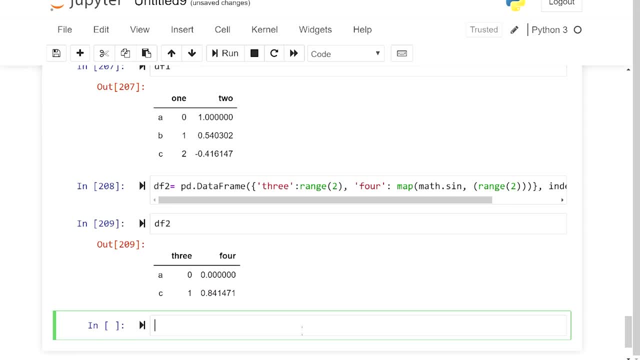 and the values. Now we want to stack these two using the concatenation technique, So pdconcat. in a list I specify which data sets, df1 and df2, and then I just define keys. For the first data, I go with level 1.. 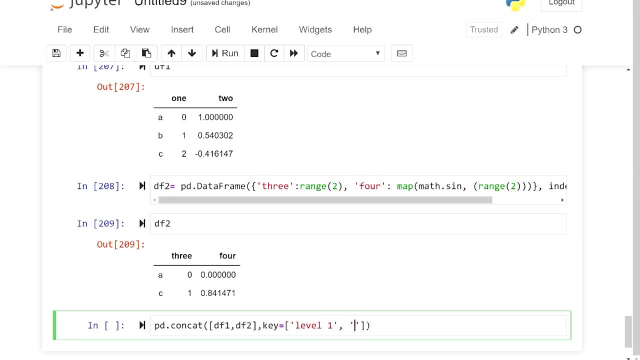 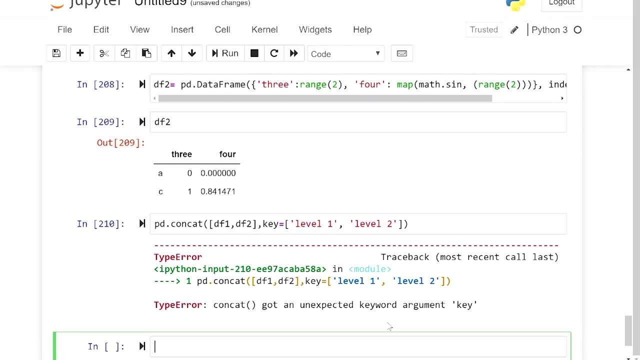 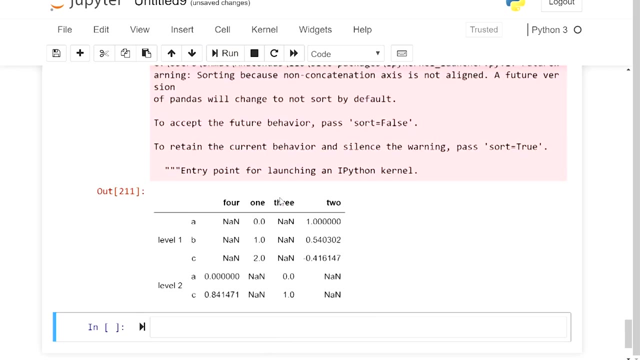 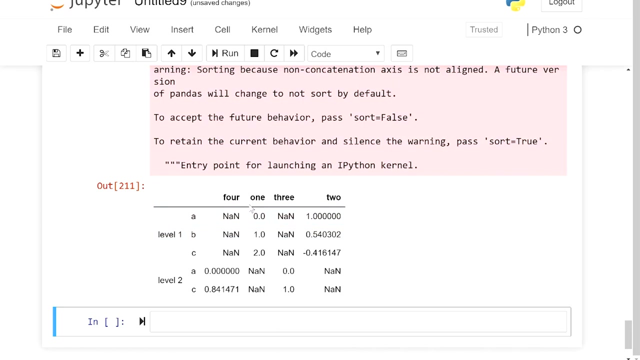 And for the second data set, df2, I go with level two. so let's run this. this is what you see. so we have a table with four columns- one, two, three and four- and then you can see the keys. level one and level two are assigned to rows and you also 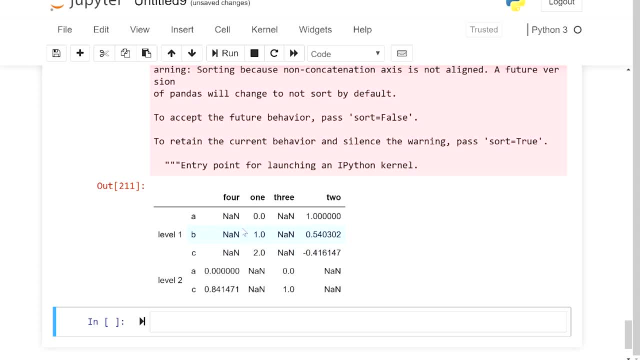 see some missing values because this method only is tax to data sets. now let's pass: X is equal to 1, then level 1 and level 2 become column headers. so I use the same method. PD can, cat, df1. so I apply to the same data set. this time I pass axis. 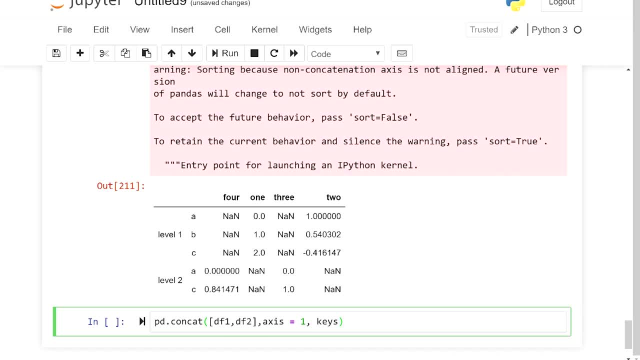 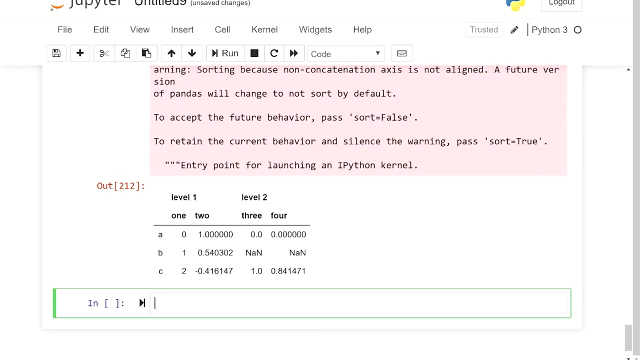 equal to 1 and keys are the same- level 1 and level 2- and now this is the result, and so for the first data set, we had 1 and 2 as the columns and level 1 as the header, and for the second data set, we had 3 and 4 and level 2 is the header for these. 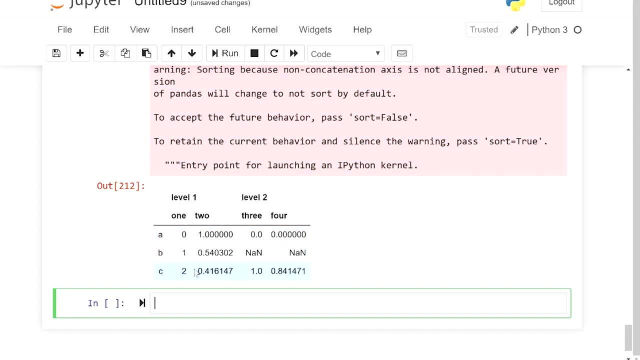 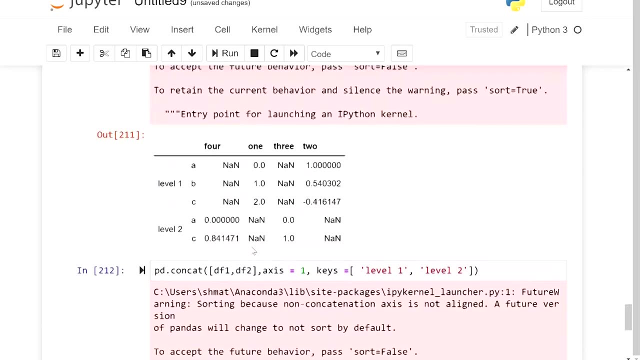 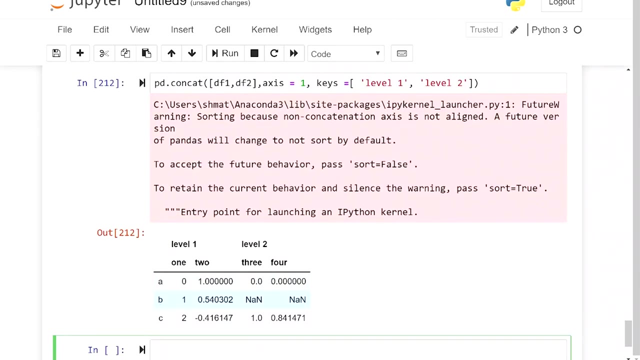 two columns and you can see three rows with two missing values. because for, if you look at the second data, so we have results for a and C and that's why for, for row B, you see missing values. because we only have values for a and C. so that's how we assigned. 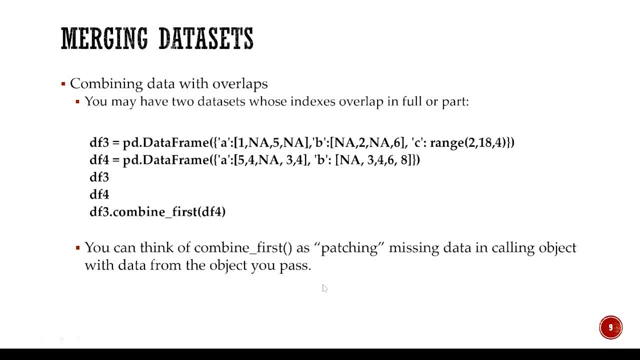 to data sets and the third method on their merging data set was combining data with overlaps and use one data set to fill in missing values in another data set so you may have to data set whose indexes overlap in full or part. then we can use combine underlying first method as a pet as patching. 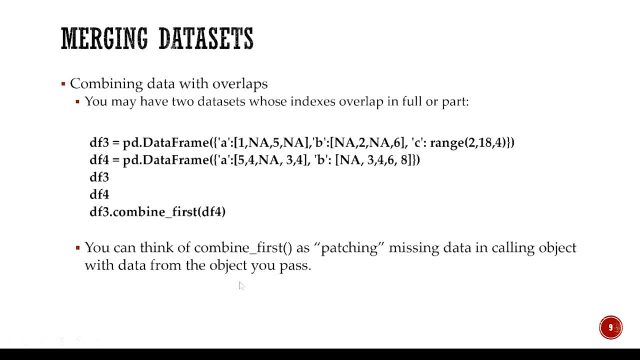 missing data in calling object with data from the object you pass. so if you look at this example, we have two data set- df3, df4, their data frame and both have some missing values, and now we want to you use one of the data set, df4 and then fill in some missing values in df3. so let's implement this and 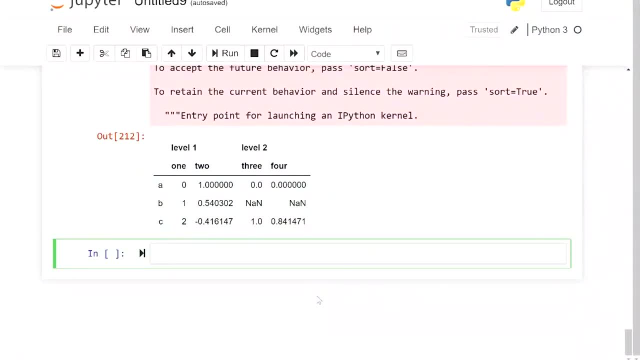 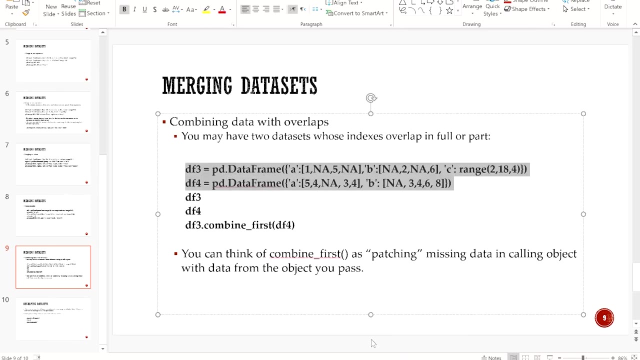 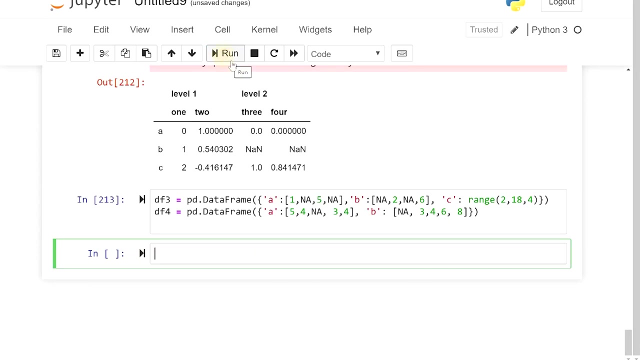 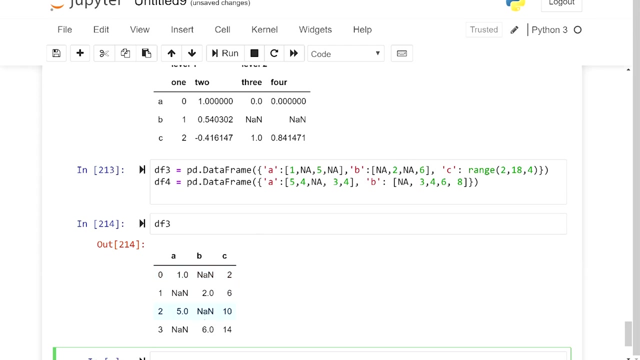 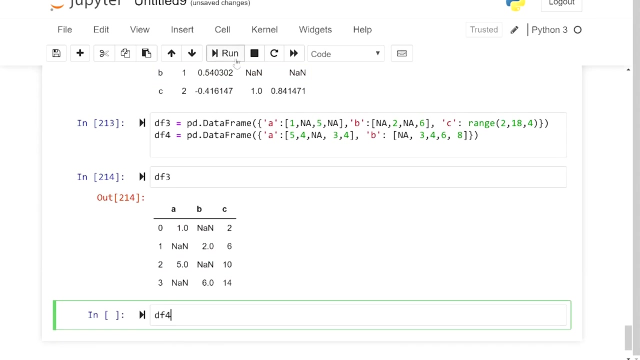 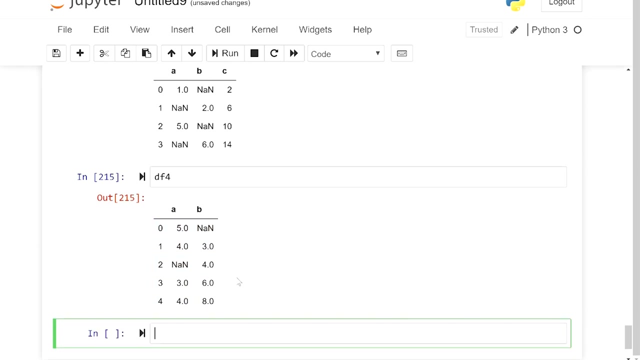 then you can see the results. df3 is a data frame. I can copy from here to make sure we don't have any typos. okay, let me print. so the first data has three columns and four rows and a few missing values. df4 has two column, five rows and some missing values, and if I apply the combine first method, I 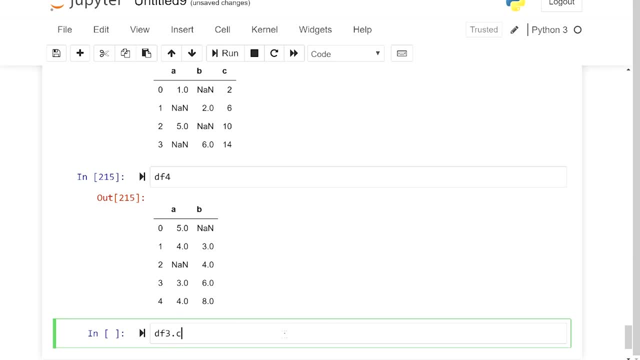 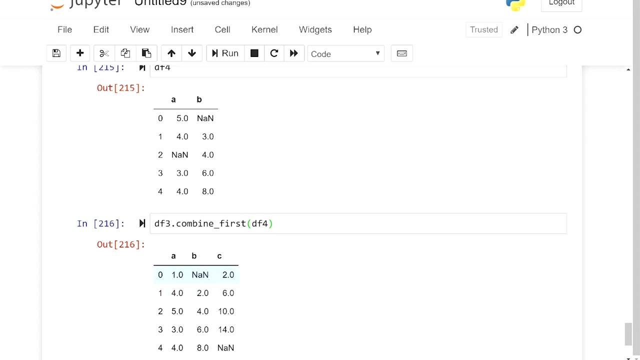 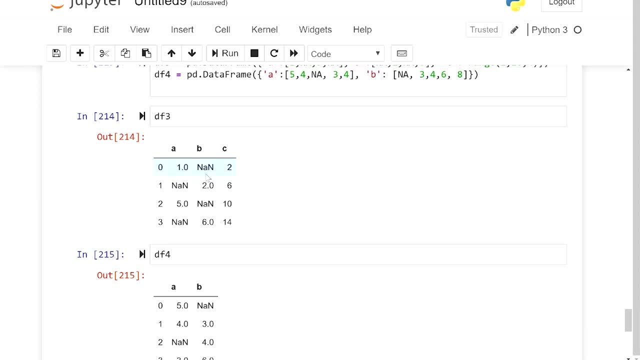 so you can see that we have ABC, three columns, five rows. so let's look at column B, B row zero. it's missing value. it's the B row- zero. it's missing value. it's the B row- zero. it's missing value. it's the same case and the second data set. so 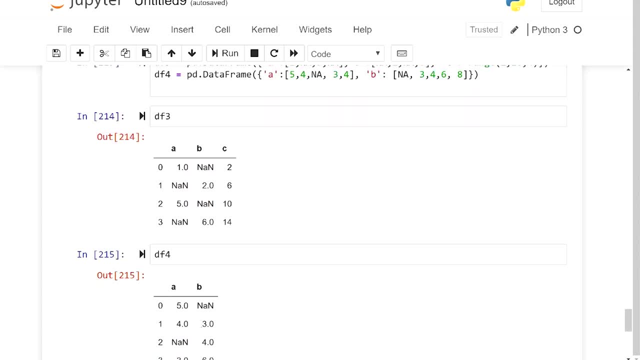 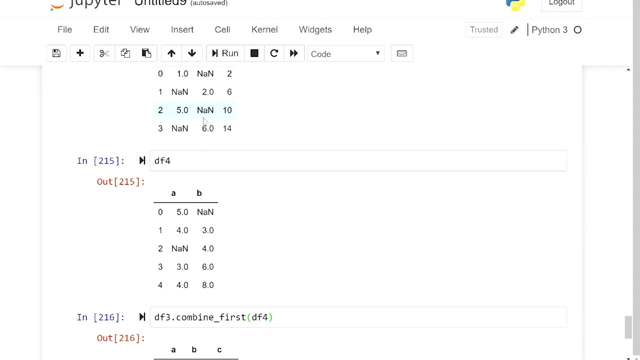 same case and the second data set. so same case and the second data set. so that's why here you still see a missing. that's why here you still see a missing. that's why here you still see a missing value. but let's look at column B, row, the 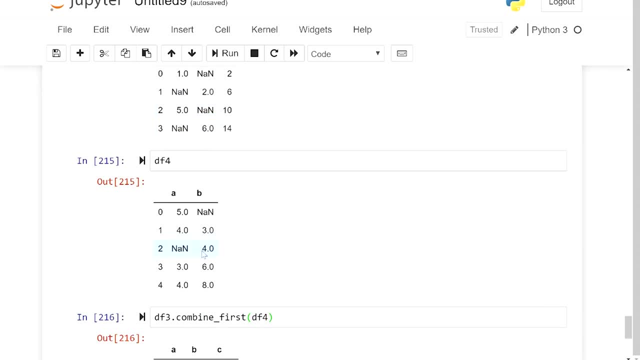 value. but let's look at column B, row, the value. but let's look at column B, row, the third row, so you see value four, and now third row, so you see value four, and now third row. so you see value four. and now four can be assigned here, the third row. 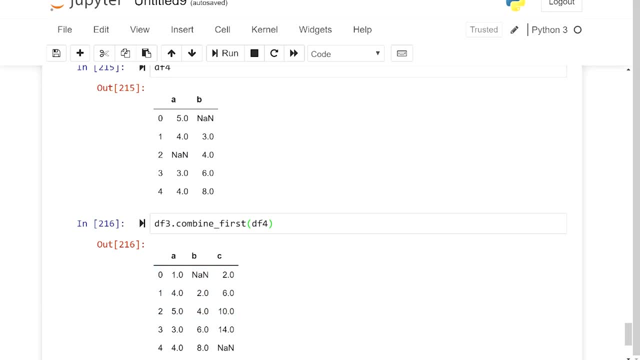 four can be assigned here. the third row four can be assigned here, the third row. for is assigned, and so that's how we can for is assigned, and so that's how we can for is assigned, and so that's how we can use this data set to fill in some. 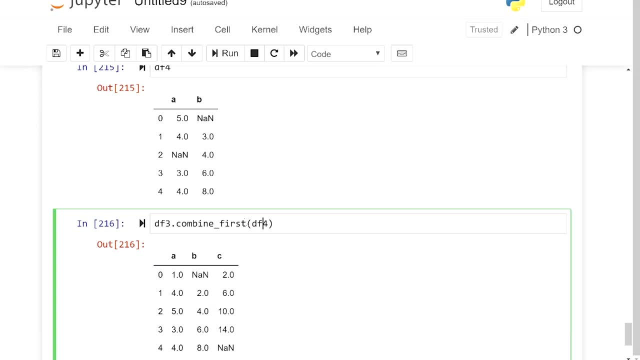 use this data set to fill in some. use this data set to fill in some missing values. if there is a value missing values. if there is a value missing values. if there is a value, otherwise it remains as a nan value, or otherwise it remains as a nan value, or. 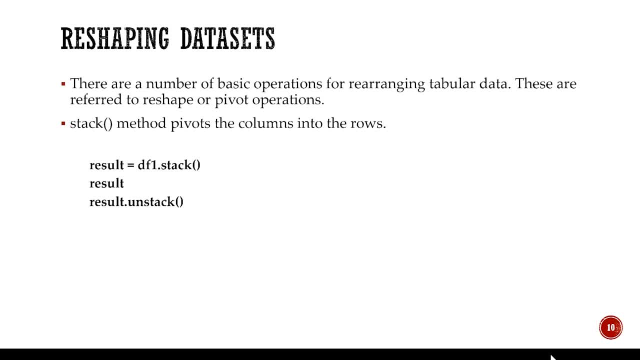 otherwise it remains as a nan value or not a number value. another useful, not a number value. another useful, not a number value. another useful technique is reshaping data set. technique is reshaping data set. technique is reshaping data set. sometimes you want to rearrange the data. 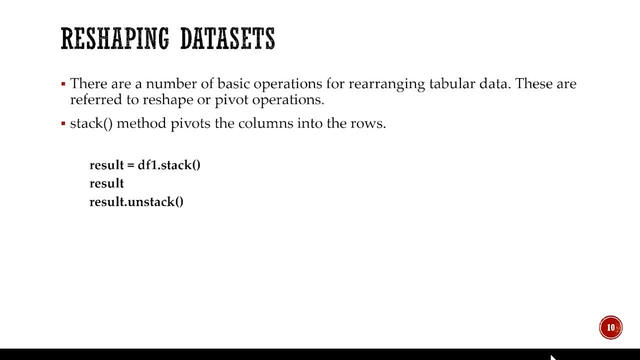 sometimes you want to rearrange the data, sometimes you want to rearrange the data and there are a number of basic and there are a number of basic and there are a number of basic operations for rearranging tabular data. operations for rearranging tabular data. 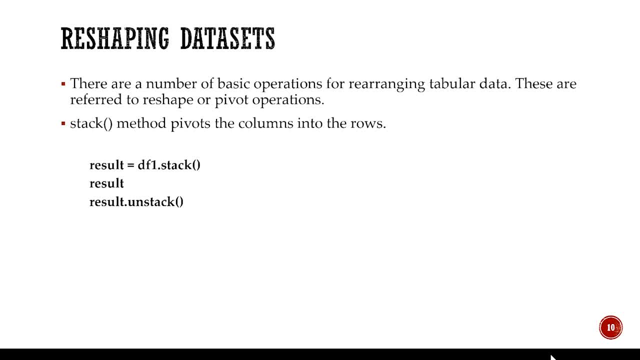 operations for rearranging tabular data, and these methods are referred to. and these methods are referred to, and these methods are referred to reshape or pivot operations. one of the reshape or pivot operations, one of the reshape or pivot operations, one of the useful method, is called a stack method. 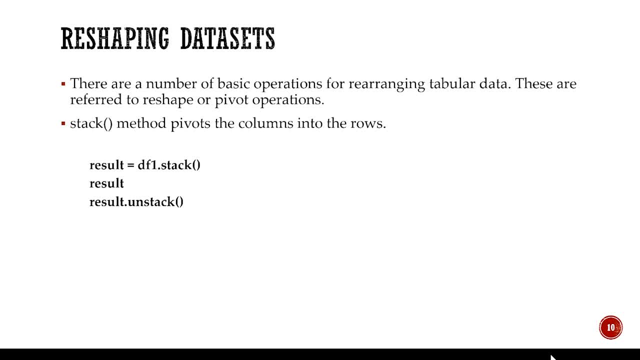 useful method is called a stack method. useful method is called a stack method which pivots the columns into the rows. which pivots the columns into the rows. which pivots the columns into the rows. it's like transposing a matrix: we change. it's like transposing a matrix: we change. 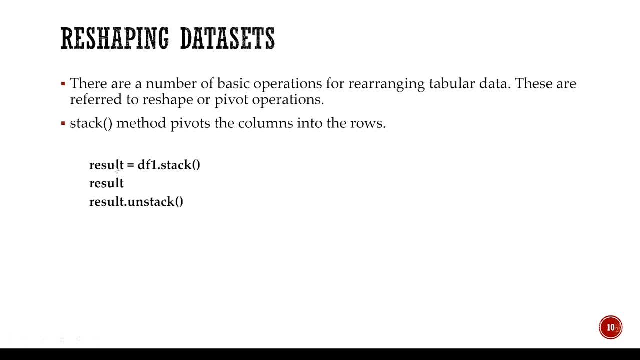 it's like transposing a matrix. we change rows and columns. in this example, we rows and columns. in this example, we rows and columns. in this example, we define another variable name result. define another variable name result. define another variable name result. we call df1 that we just 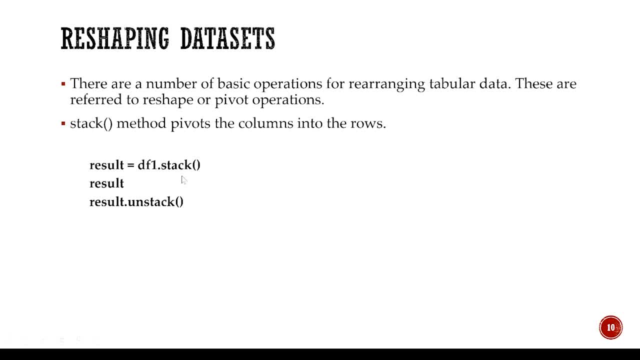 we call df1 that we just we call df1 that we just created, then we apply the stack method created, then we apply the stack method created, then we apply the stack method, then, then, then it should um change the rows and it should um change the rows and. 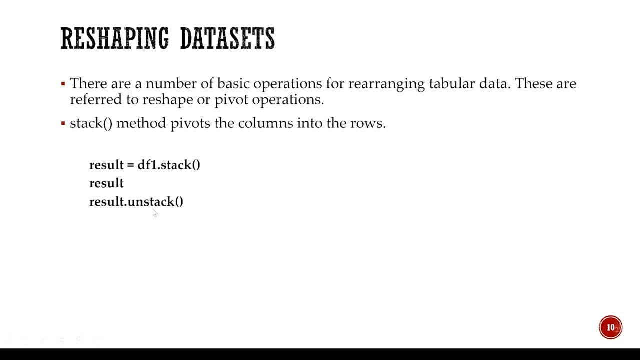 it should um change the rows and columns, columns, columns, and if you want to undo, and if you want to undo, and if you want to undo what you just did, then you call the on what you just did, then you call the on what you just did, then you call the on stack method, then you should see the. 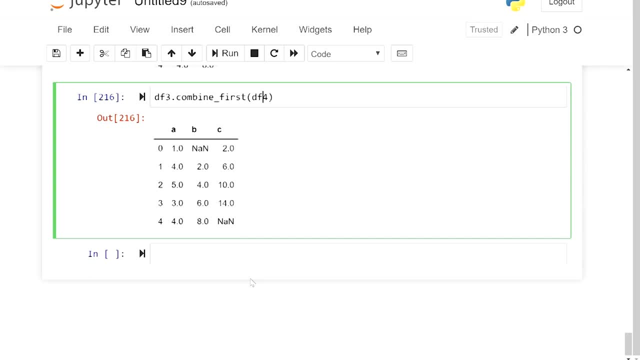 stack method, then you should see the stack method. then you should see the original data state. original data state. original data state. let's implement this and see what the let's implement this and see what the let's implement this and see what the results look like. results look like. 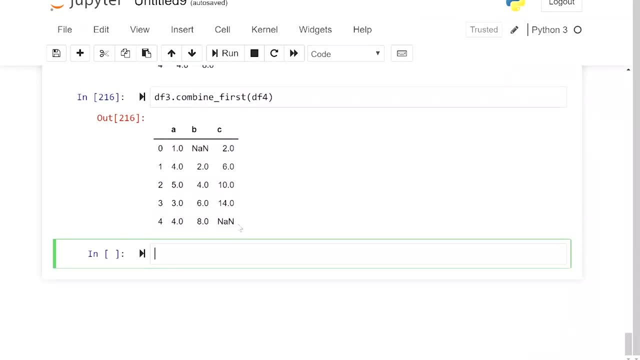 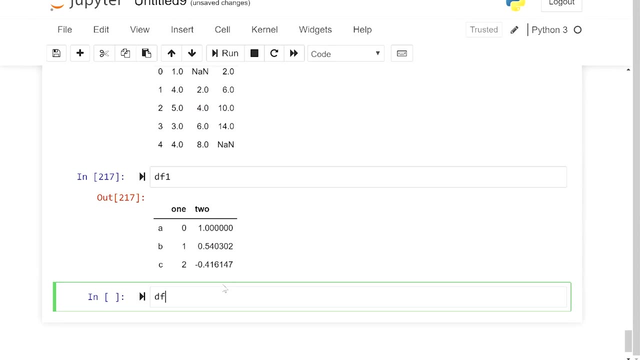 results look like: so df1 is referring. let me print this. so df1 is referring. let me print this. so df1 is referring. let me print this. this is df1. this is df1. this is df1. and now if we apply. and now, if we apply. 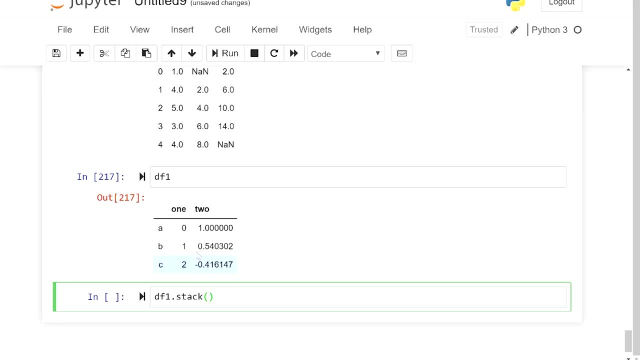 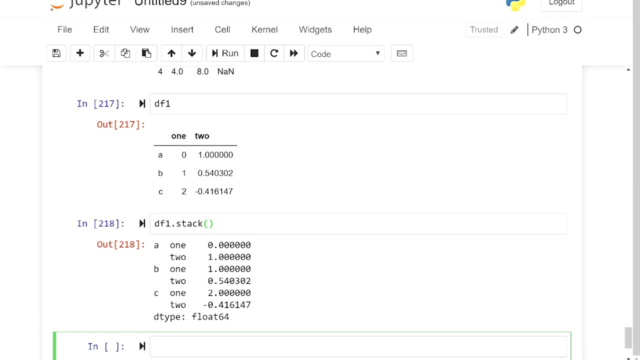 and now, if we apply the stack method, the stack method, the stack method, so it has three rows, two columns, and now you can see, and now you can see, and now you can see, it changes it, changes it, changes the rows and columns it, the rows and columns it. 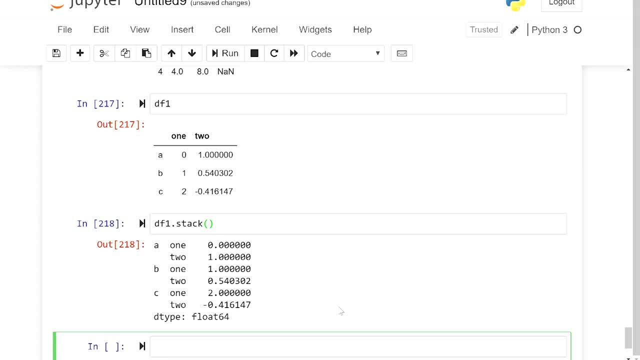 the rows and columns, it rearranges, rearranges, rearranges the data in a tabular format. and now if the data in a tabular format? and now if the data in a tabular format? and now, if we apply the on a stack, we apply the on a stack. 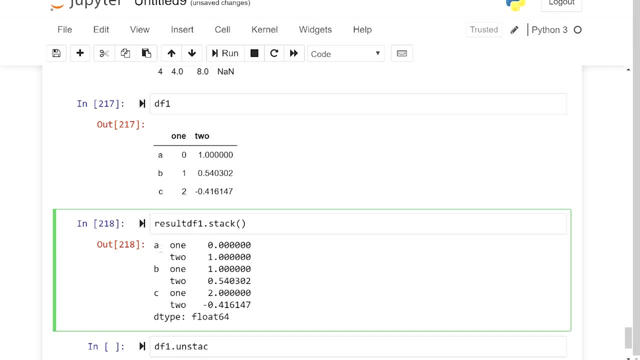 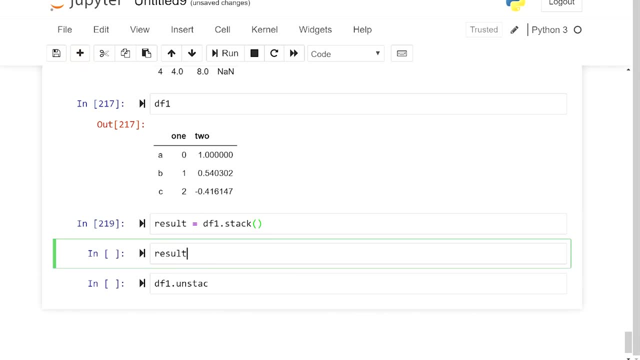 we apply the on a stack, so let me save this in a variable. so result: now this would be the. now this would be the. now this would be the so one, two. you can see that now they so one, two. you can see that now they so one, two. you can see that now they are in. 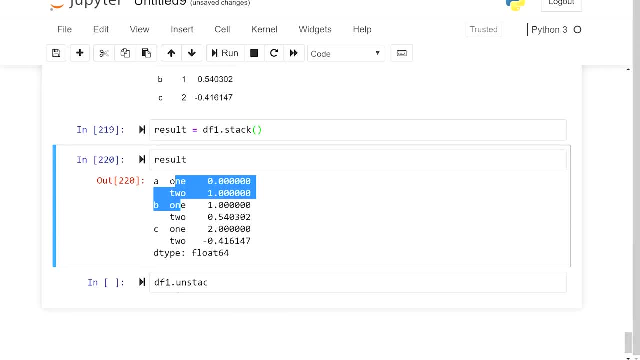 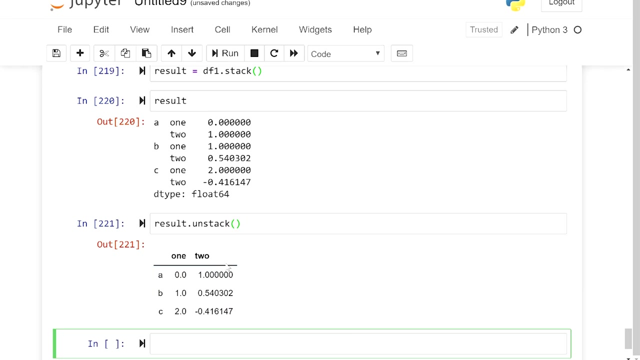 are in, are in each row, and the values here, each row, and the values here, each row, and the values here. now we apply the on stack method and then we have the original data frame. so that's one, uh, one of the data frame. so that's one, uh, one of the. 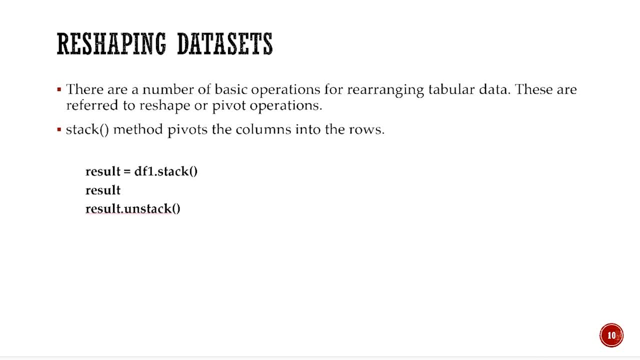 data frame. so that's one, uh one, of the useful techniques for rearranging, useful techniques for rearranging, useful techniques for rearranging or reshaping your data set, or reshaping your data set, or reshaping your data set. so with this example, we wrap up our so with this example, we wrap up our. so with this example, we wrap up our discussion on data rank. discussion on data rank.